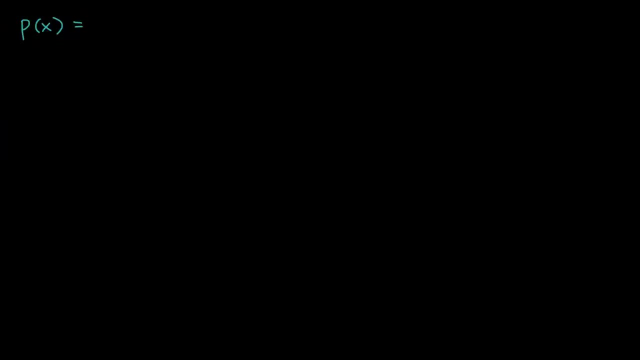 Let's say that we have a polynomial p of x and we can factor it and we can put it in the form x minus one times x plus two times x minus three times x plus four, And what we are concerned with are the zeros of this polynomial. 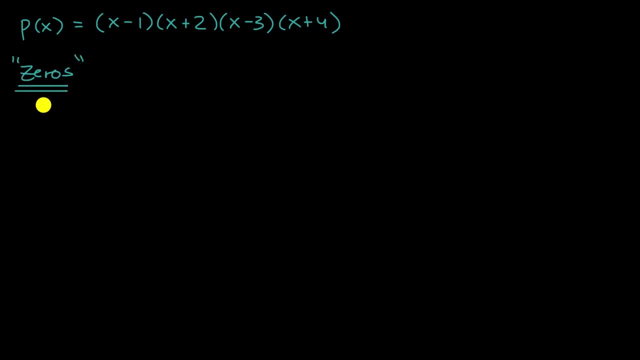 And you might say: what is a zero of a polynomial? Well, those are the x values that are going to make the polynomial equal to zero. So another way to think about it is: for what x values is p of x going to be equal to zero? 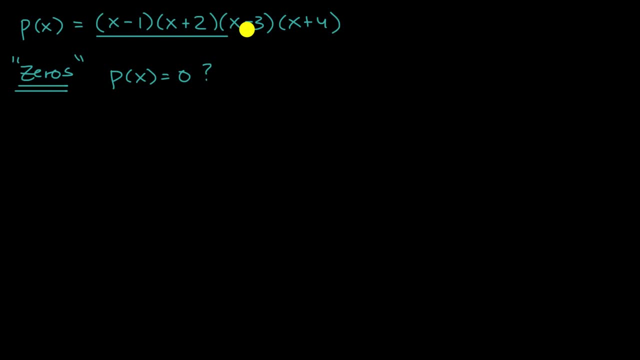 Or another way you can think about it is: for what x values is this expression going to be equal to zero. So for what x values is x minus one times x plus two times x minus three times x plus four going to be equal to zero? 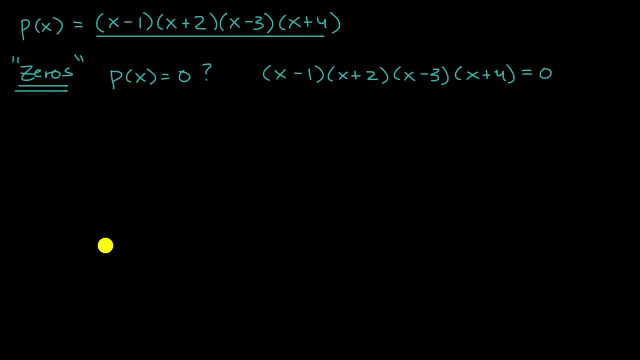 I encourage you to pause this video and think about that a little bit before we work through it together. Well, the key realization here is: if you have the product of a bunch of expressions, if any one of them is equal to zero, it doesn't matter what the others are. 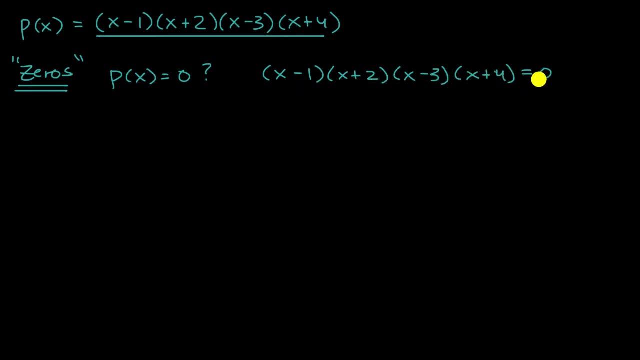 because zero times anything else is going to be equal to zero. So the fancy term for that is the zero product property. But all it says is: hey, if you can find an x value that makes any one of these expressions equal to zero. 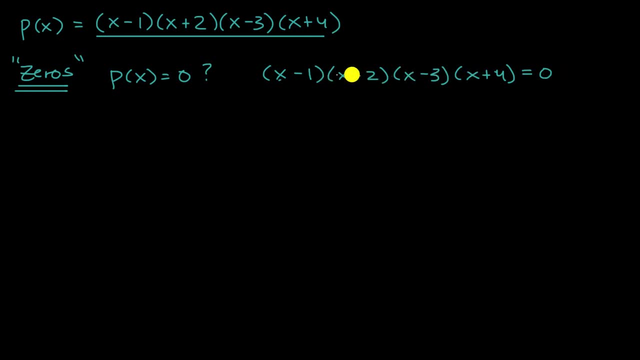 well, that's going to make the entire expression going to be. it's going to make the entire expression equal to zero. So the zeros of this polynomial are going to be the x values that could make x minus one equal to zero. So x minus one equals zero. 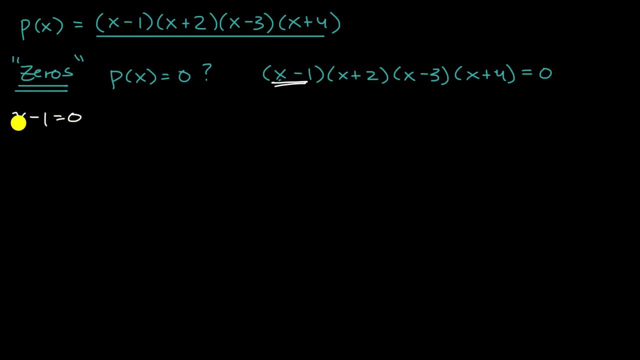 Well, we know what x value would make that happen if x is equal to one. If you add one to both sides here, x equals one, So x equals one is a zero of this polynomial. Another way to say that is p of one when x equals one. 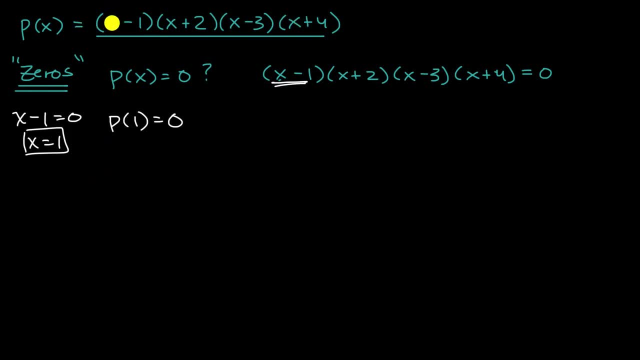 that whole polynomial is going to be equal to zero. How do I know that? Well, if I put a one in: right over here, this expression, right over here, this expression, right here, this expression, right here, this expression, right here. 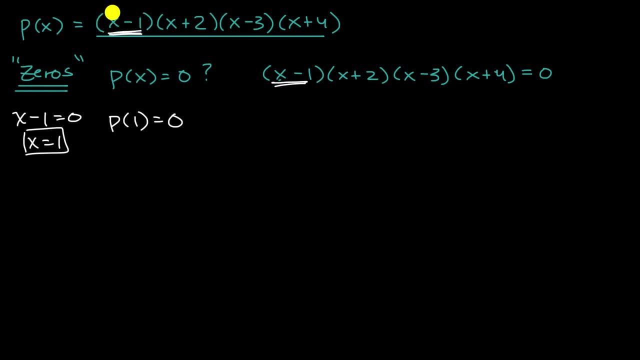 right over here: x minus one, that is going to be equal to zero. So you're gonna have zero times, a bunch of other stuff which is going to be equal to zero, And so, by the same idea, we can figure out what the other zeros are. 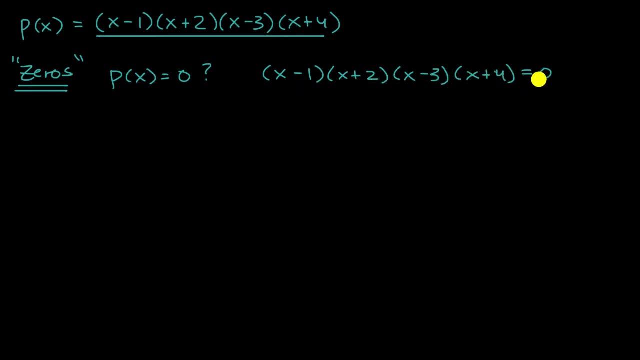 because zero times anything else is going to be equal to zero. So the fancy term for that is the zero product property. But all it says is: hey, if you can find an x value that makes any one of these expressions equal to zero. 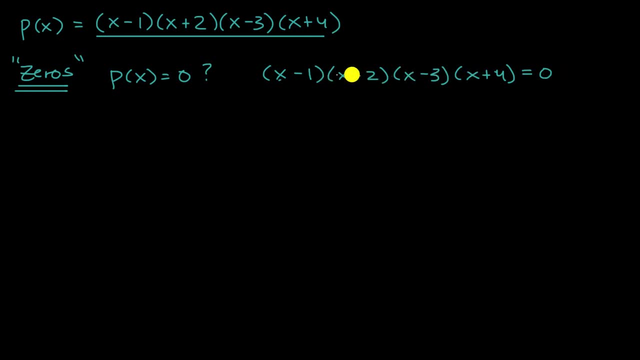 well, that's going to make the entire expression going to be. it's going to make the entire expression equal to zero. So the zeros of this polynomial are going to be the x values that could make x minus one equal to zero. So x minus one equals zero. 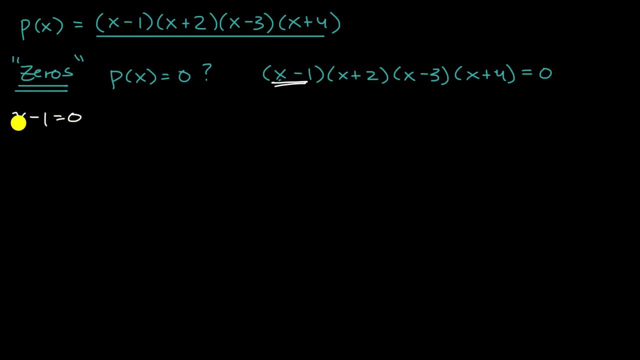 Well, we know what x value would make that happen if x is equal to one. If you add one to both sides here, x equals one, So x equals one is a zero of this polynomial. Another way to say that is p of one when x equals one. 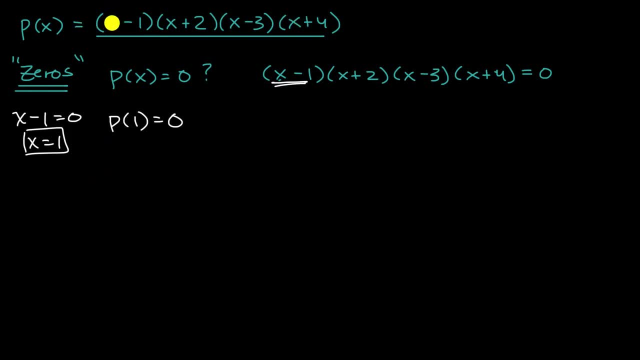 that whole polynomial is going to be equal to zero. How do I know that? Well, if I put a one in: right over here, this expression, right over here, this expression, right here, this expression, right here, this expression, right here. 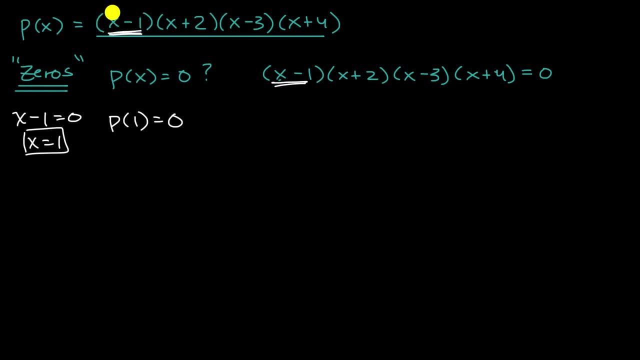 right over here: x minus one, that is going to be equal to zero. So you're gonna have zero times, a bunch of other stuff which is going to be equal to zero, And so, by the same idea, we can figure out what the other zeros are. 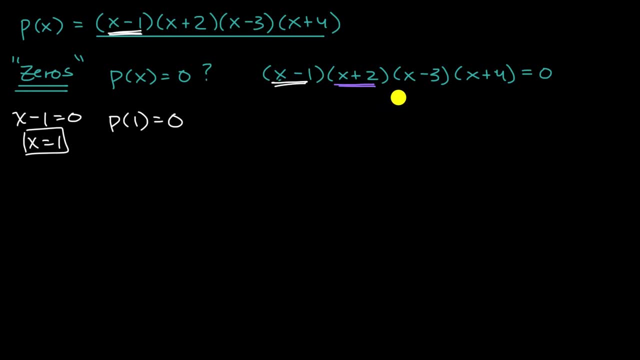 What would make this part equal to zero? What x value would make x plus two equal to zero? Well, x equals negative two. X equals negative two would make x plus two equal zero. So x equals negative two is another zero of this polynomial. 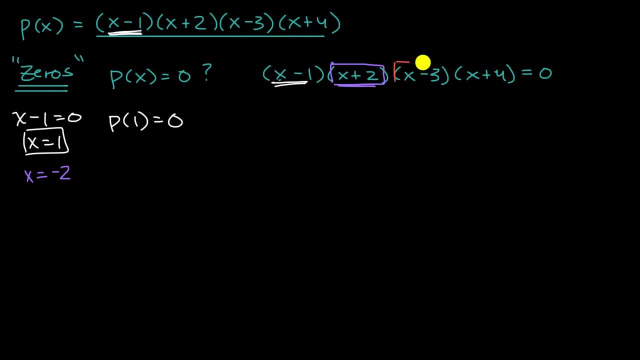 And we could keep going. What would make x minus three equal to zero? Well, if x is equal to three, that would make x minus three equal to zero, and that would then make the entire expression equal to zero. And then, last but not least, 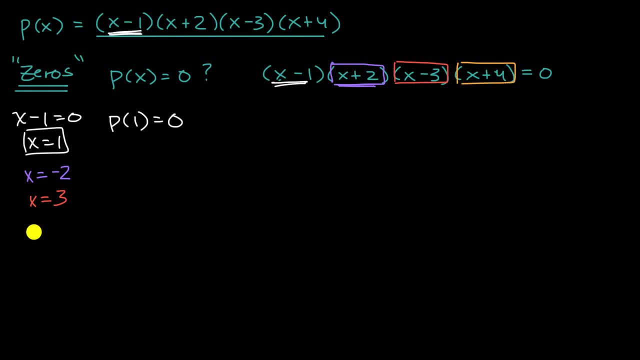 what would make x plus four equal to zero? Well, if x is equal to negative four, And just like that, we have found four zeros for this polynomial. When x equals one, the polynomial is equal to zero. When x equals negative two. 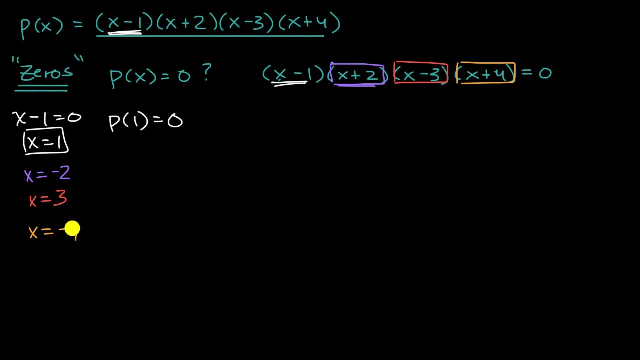 the polynomial is equal to zero. When x equals three, the polynomial is equal to zero. And when x equals negative four, the polynomial is equal to zero. And one of the interesting things about the zeros of a polynomial: you could actually use that to start to sketch out. 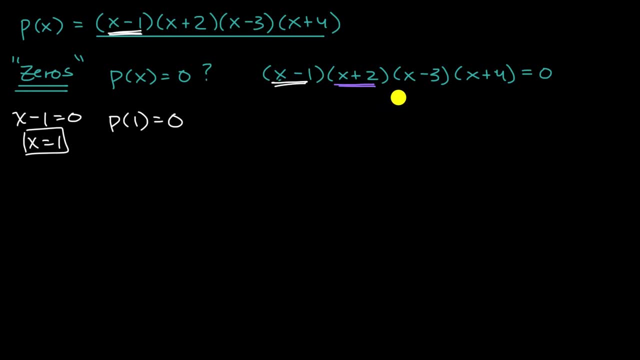 What would make this part equal to zero? What x value would make x plus two equal to zero? Well, x equals negative two. X equals negative two would make x plus two equal zero. So x equals negative two is another zero of this polynomial. 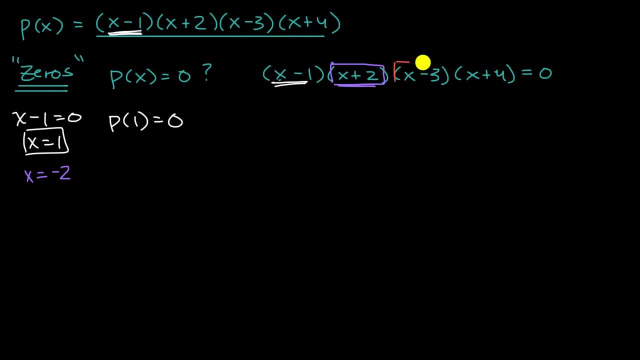 And we could keep going. What would make x minus three equal to zero? Well, if x is equal to three, that would make x minus three equal to zero, and that would then make the entire expression equal to zero. And then, last but not least, 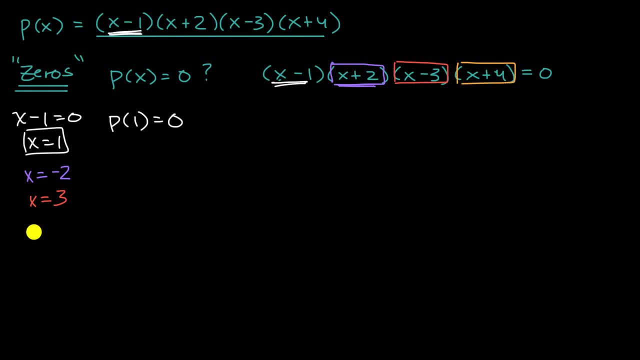 what would make x plus four equal to zero? Well, if x is equal to negative four, And just like that, we have found four zeros for this polynomial. When x equals one, the polynomial is equal to zero. When x equals negative two. 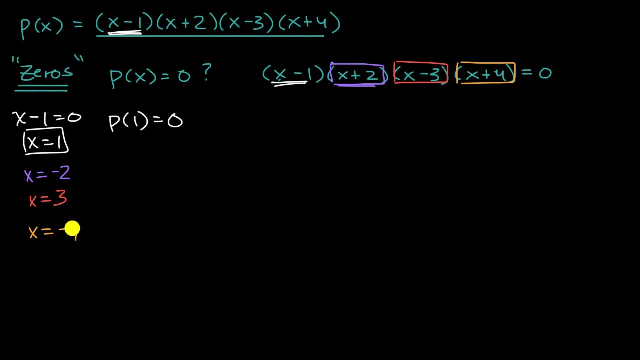 the polynomial is equal to zero. When x equals three, the polynomial is equal to zero. And when x equals negative four, the polynomial is equal to zero. And one of the interesting things about the zeros of a polynomial: you could actually use that to start to sketch out. 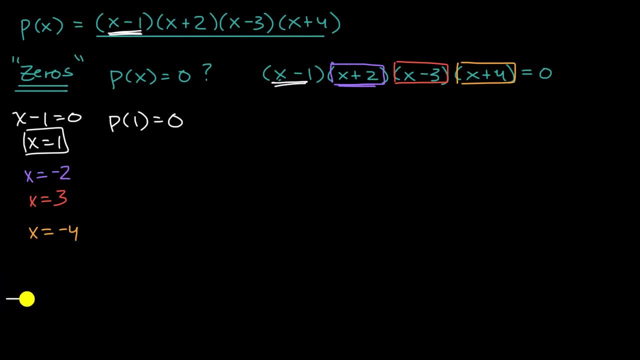 what the graph might look like. So, for example, we know that this polynomial is going to take on the value zero at these zeros. So let me just draw a rough sketch right over here. So if this is my x-axis, that's my y-axis. 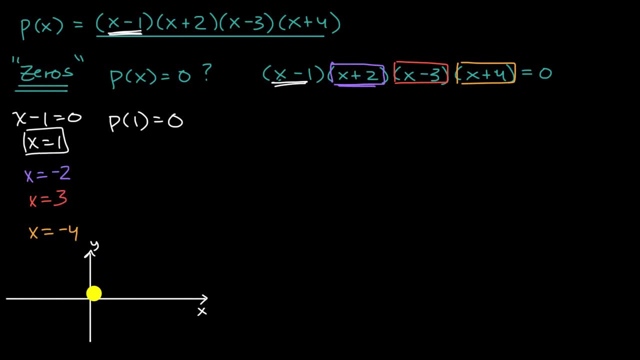 So that's my y-axis, And so let's see, At, x equals one, so let me just do it this way. So we have one, two, three and four, And then you have negative one, negative two, negative, three. 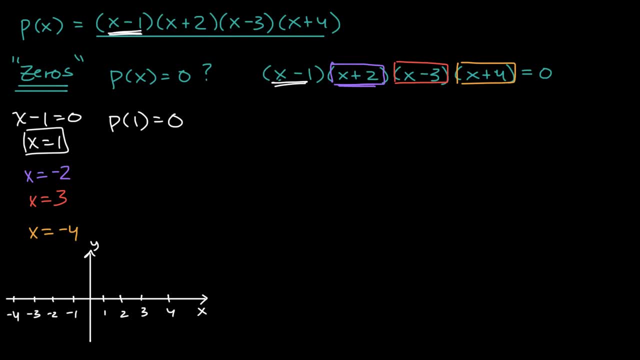 and then, last but not least, negative four. We know that this polynomial p of x is going to be equal to zero at x equals one, So it's going to intersect the x-axis right there. It's going to be equal to zero at x equals negative two. 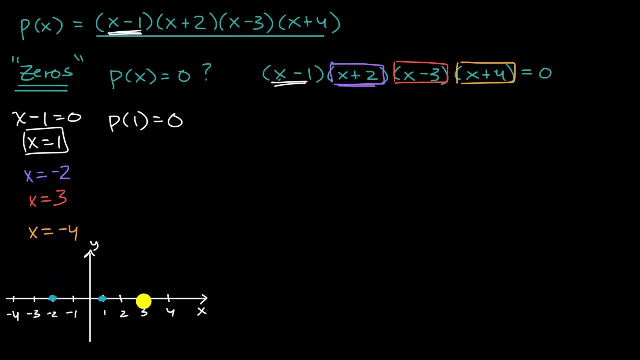 so right over there At x equals three right over there, And x equals negative four. Now we don't know exactly what the graph looks like. just based on this, We could try out some values on either side to figure out. hey, is it above the x-axis? 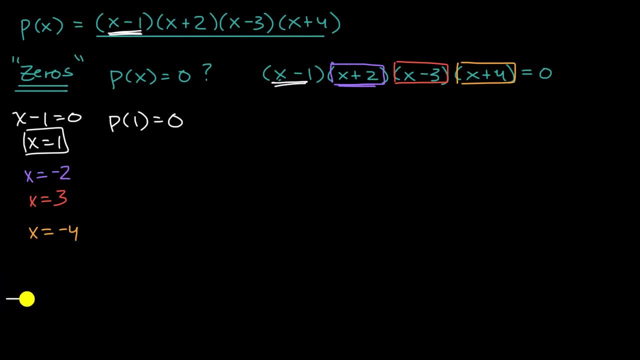 what the graph might look like. So, for example, we know that this polynomial is going to take on the value zero at these zeros. So let me just draw a rough sketch right over here. So if this is my x-axis, that's my y-axis. 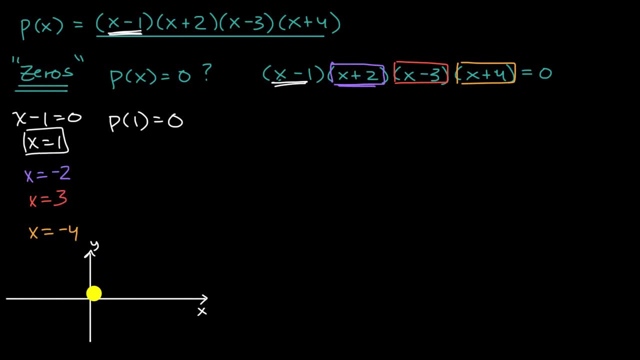 So that's my y-axis, And so let's see, At, x equals one, so let me just do it this way. So we have one, two, three and four, And then you have negative one, negative two, negative, three. 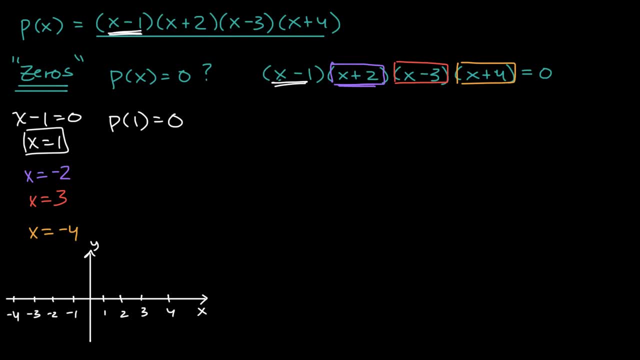 and then, last but not least, negative four. We know that this polynomial p of x is going to be equal to zero at x equals one, So it's going to intersect the x-axis right there. It's going to be equal to zero at x equals negative two. 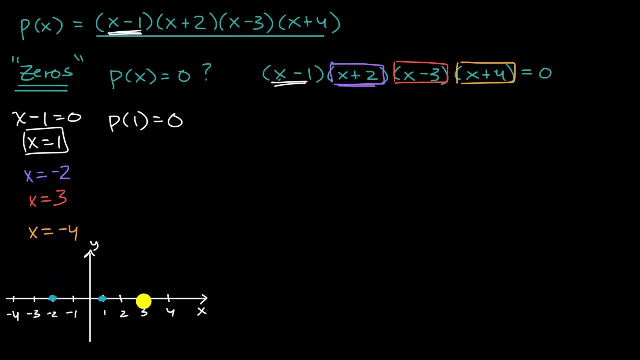 so right over there At x equals three right over there, And x equals negative four. Now we don't know exactly what the graph looks like. just based on this, We could try out some values on either side to figure out. hey, is it above the x-axis? 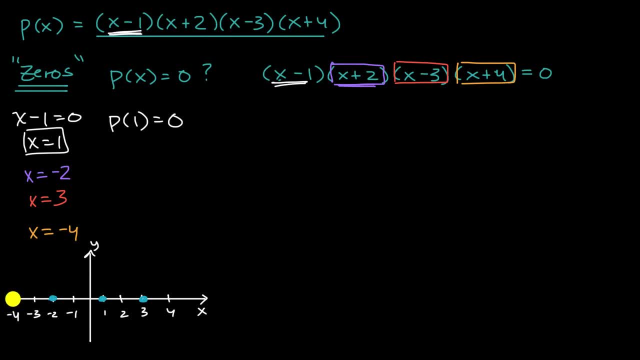 or below the x-axis for x values less than negative four, And we can try things out like that, but we know it intersects the x-axis at these points, So it might look something like this. This is a very rough sketch. It might look something like this: 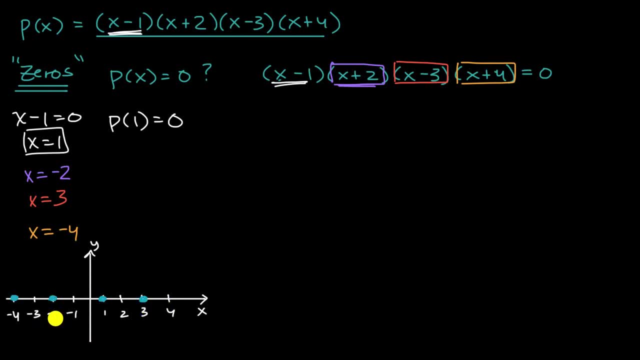 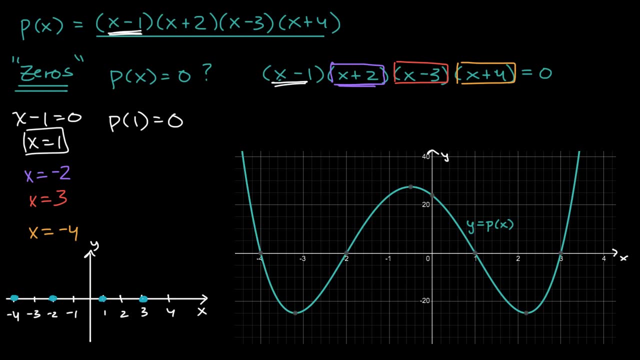 We don't know Without doing a little bit more work, But ahead of time I took a look at what this looks like. I went on to Desmos and I graphed it And you can see it looks exactly as what we would expect. 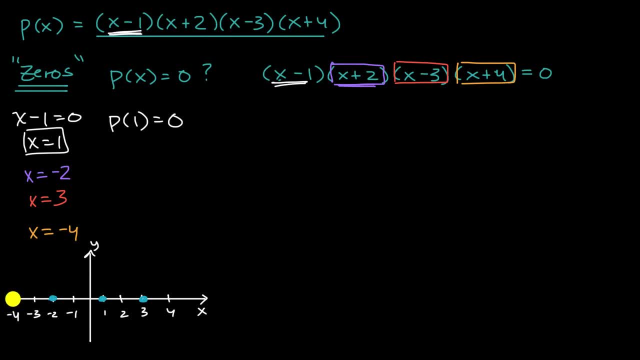 or below the x-axis for x values less than negative four, And we can try things out like that, but we know it intersects the x-axis at these points, So it might look something like this. This is a very rough sketch. It might look something like this: 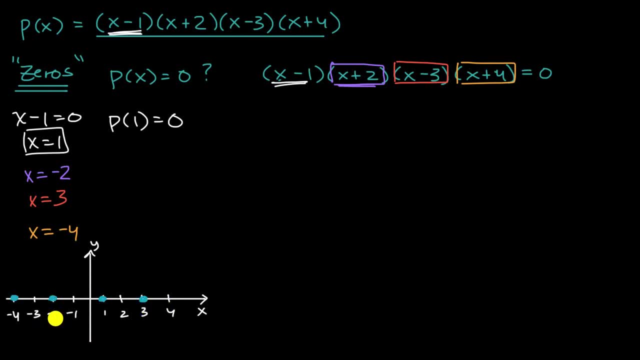 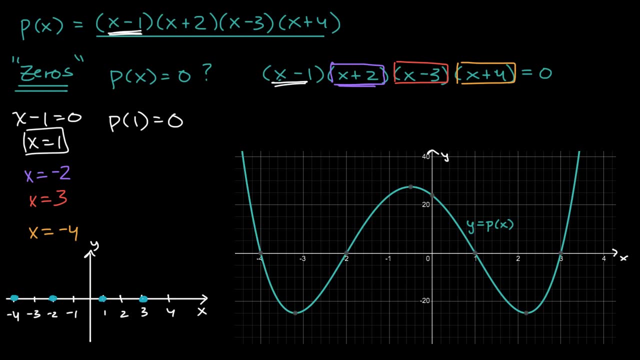 We don't know Without doing a little bit more work, But ahead of time I took a look at what this looks like. I went on to Desmos and I graphed it And you can see it looks exactly as what we would expect. 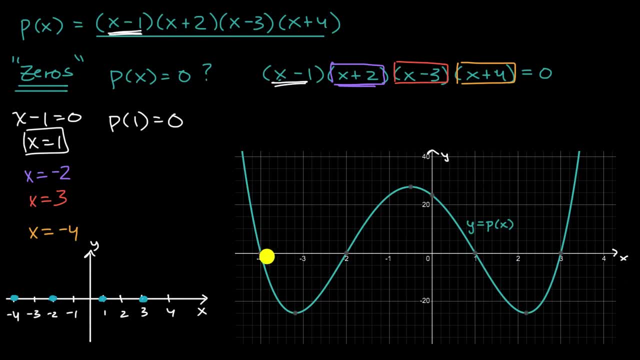 The graph of this polynomial intersects the x-axis at. x equals negative four. Actually, let me color code it: X equals negative four, and that is that zero right over there. X equals negative two. that's this, zero right there. X equals one right over there. 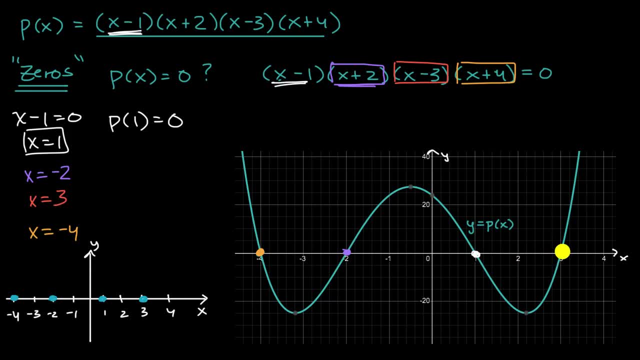 And then x equals three right over there. In future videos, we will study this in even more depth. 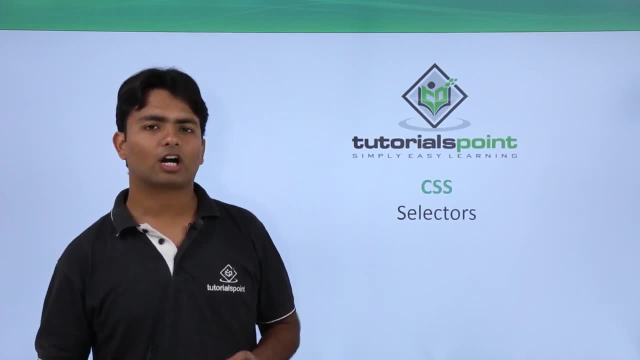 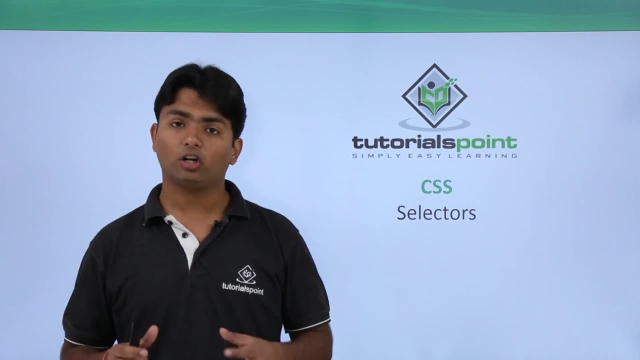 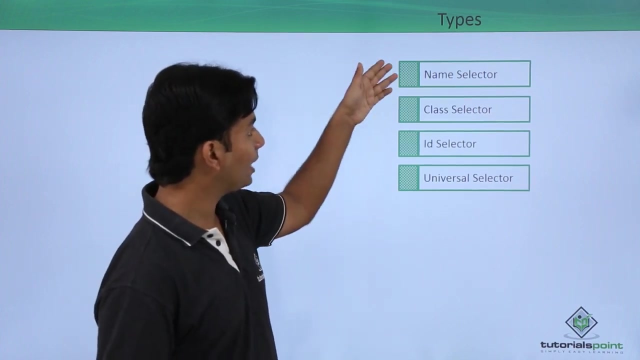 Hi, now in this video of CSS we will talk about the selectors. Selectors are basically something which will help us out in selecting the particular element or the particular portion of your web page. So here we have four kinds of basic selectors. These are: name selector, class selector id. 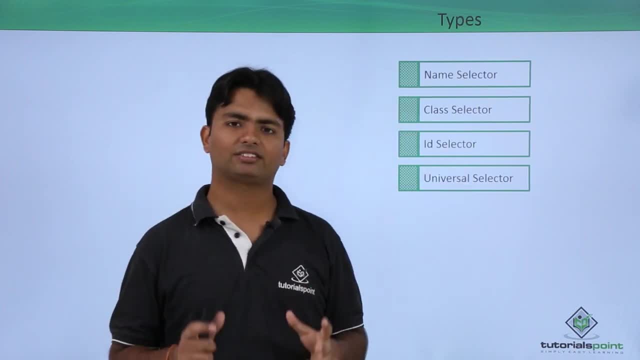 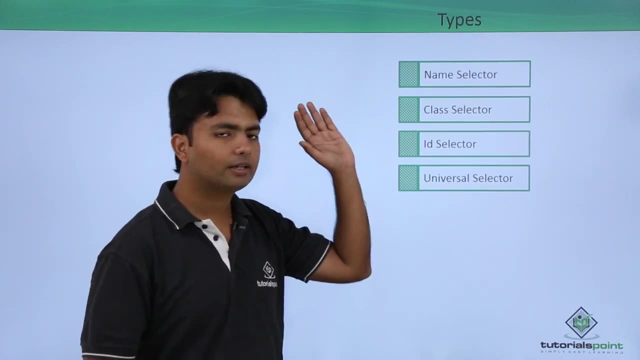 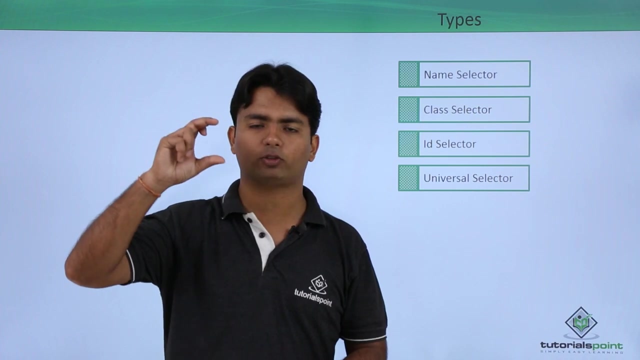 selector and universal selector. The name selector is something where you will pass the name of the particular tag for which you want to apply the styles. For example, if I want to make some styles for the heading h1 or h2, I will use h2 as the name of the tag and inside this I will put all. 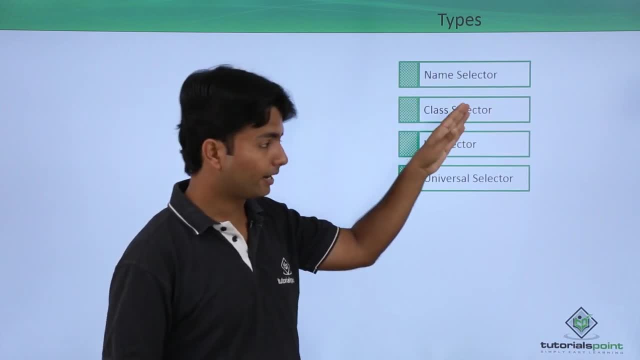 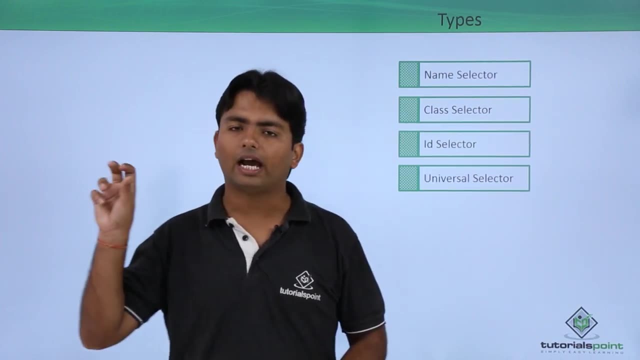 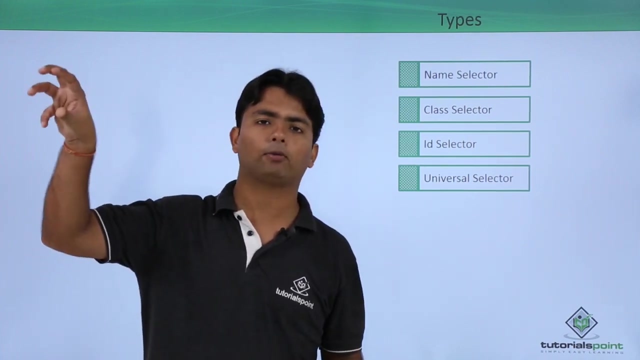 these styles which I want to put for that particular tag. Now, second is the class selector, where I will put dot as a class selector and that particular class of CSS will contain some list of styles. When, On a document, I want to apply that particular set of styles to a particular element, I will use the